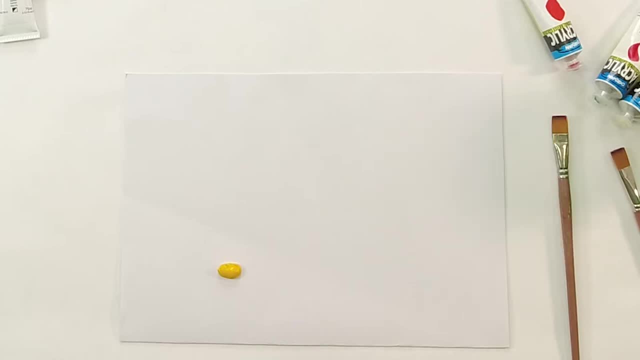 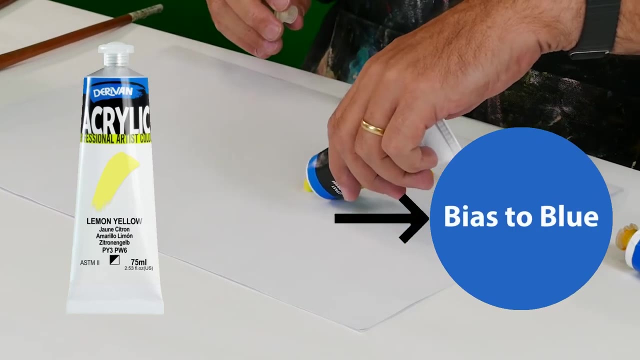 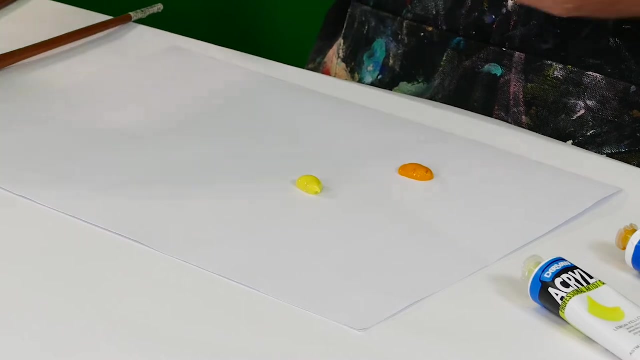 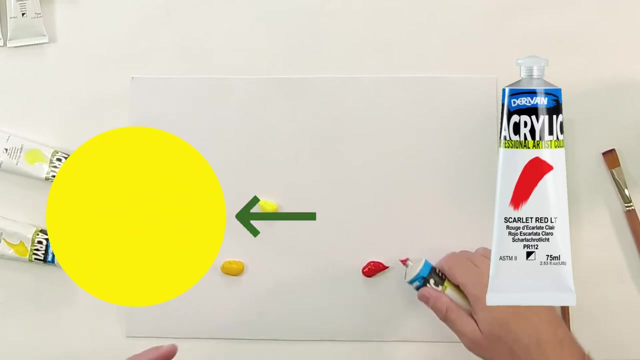 biased towards red, the yellow, as opposed to lemon yellow, And I'll show you what sort of orange we get with that in a second. And then we're going to use scarlet, which is a very yellowy red. So it's biased towards the yellow, And out of that we're going to 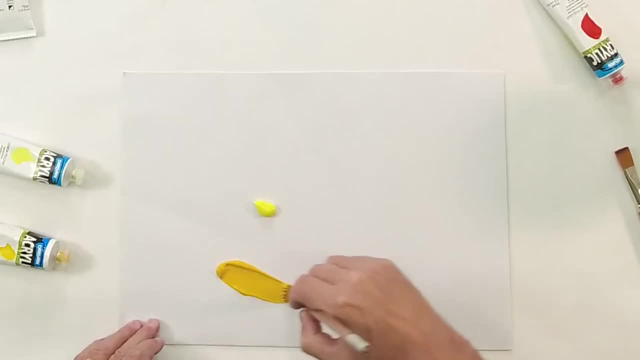 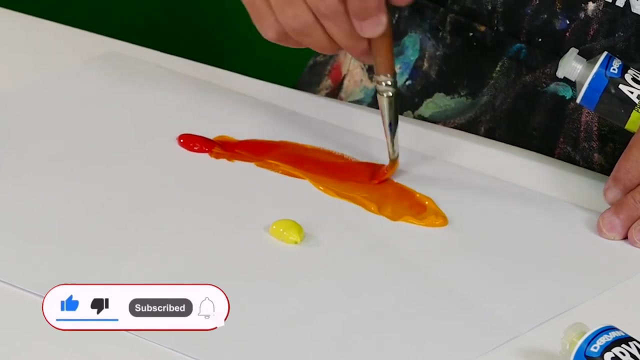 mix. We're not going to use a purple, We're going to mix a yellow, And then we're going to use a palette knife. We're just going to grab some of this like this, mix it around, pick up a little bit of the red And there we've got a nice vibrant yellow orange even. 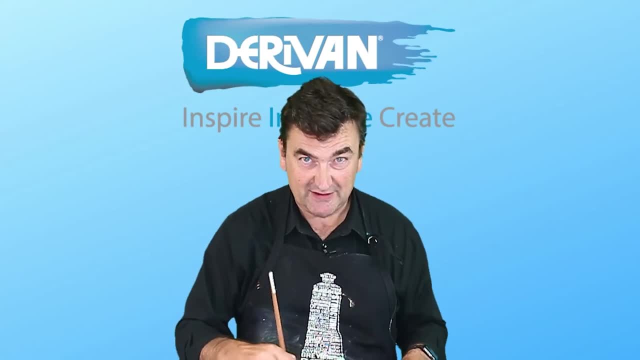 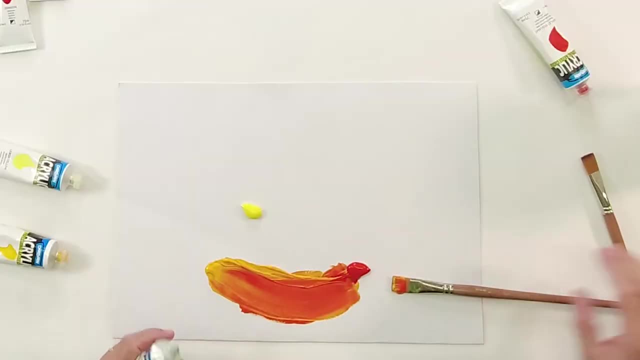 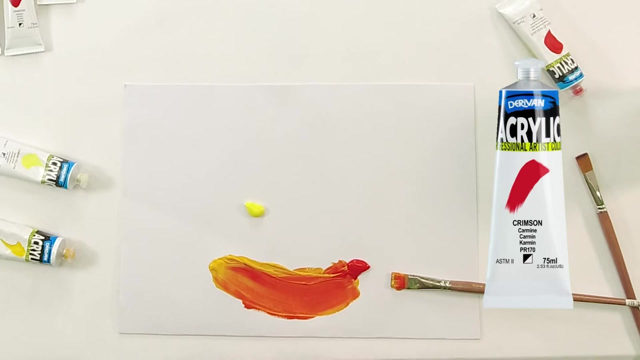 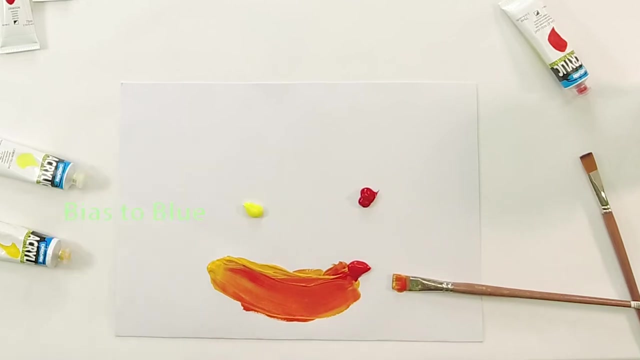 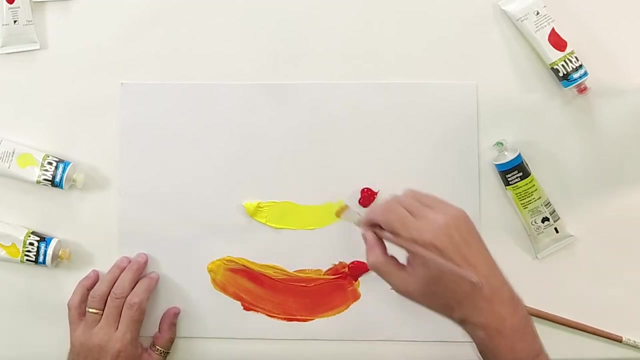 Any idea what rhymes with orange? We'll tell you later, Maybe. So we've got a nice, Nice, bright orange. Now if I take a crimson, which is a very blue or a very cool red, and mix that with a very blue or lemon yellow, I'll get an orange as well. But as you'll 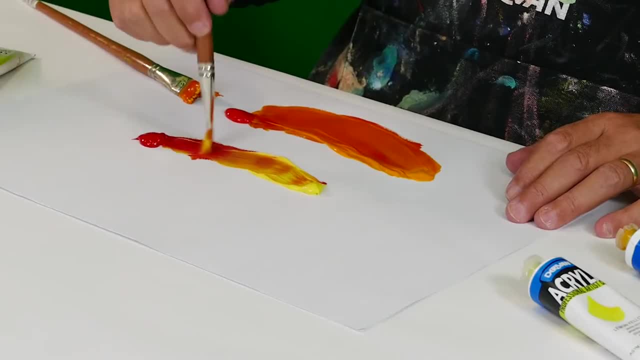 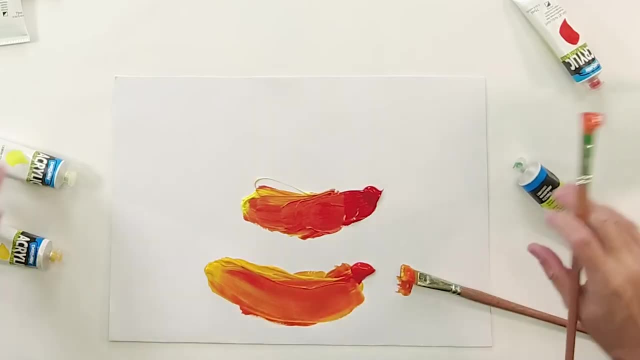 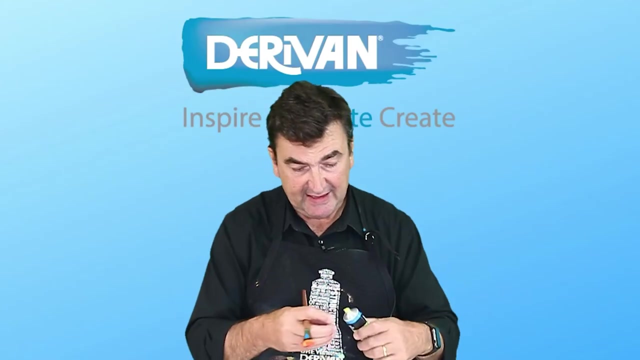 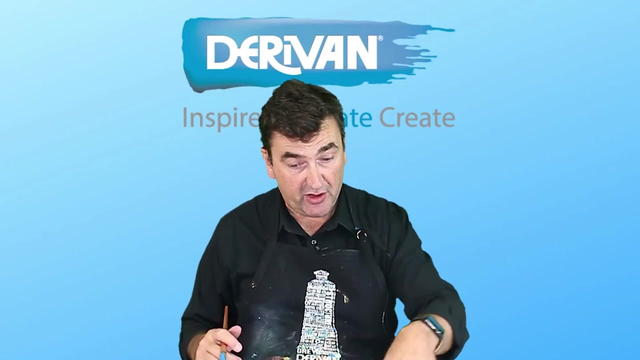 see, it'll be quite a deep, Dirty orange, Much dirtier than this nice bright orange. here I might use a little bit more yellow, And the reason that is is because we have more of our third primary, the blue. 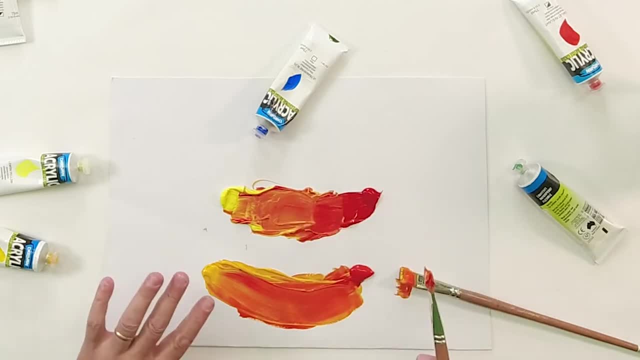 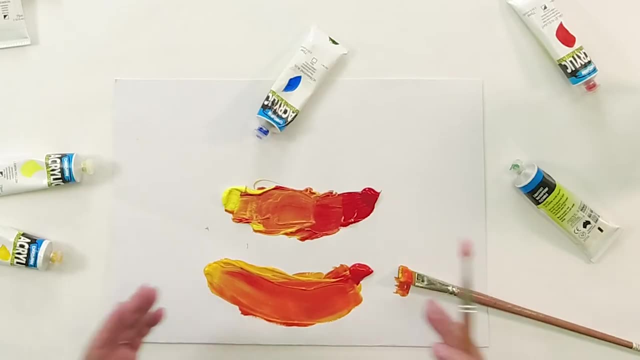 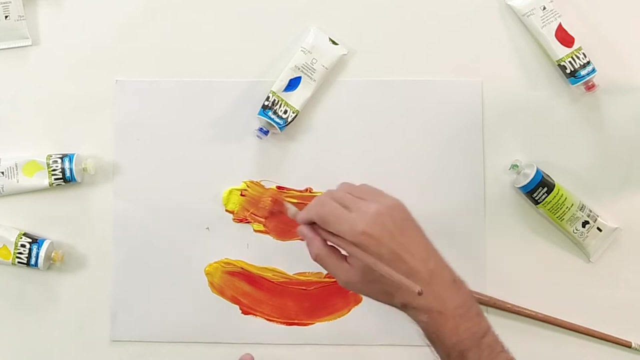 in these two colours than we do in these two colours. So, as we said before, the yellow, So as we said before the yellow: The yellow deep is a red-leaning yellow and the scarlet is a yellow-leaning red. So we're keeping that third primary out which gives us this beautiful, clean, bright, vibrant.